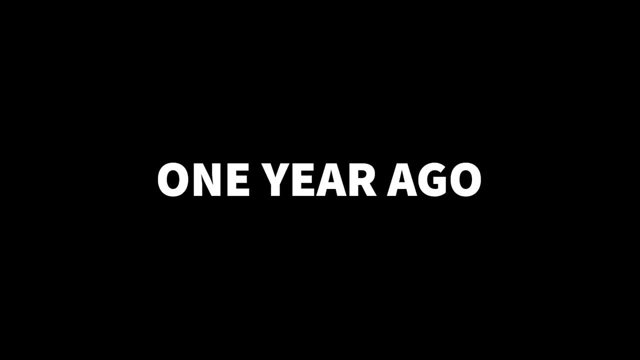 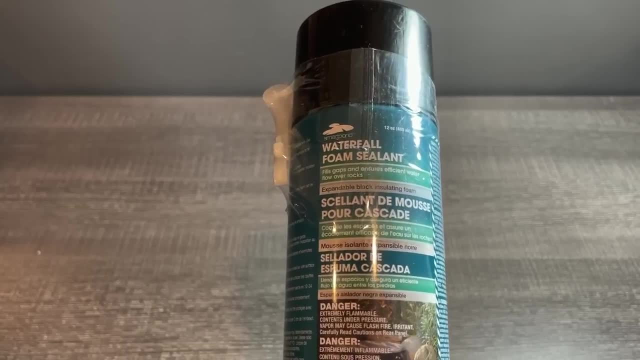 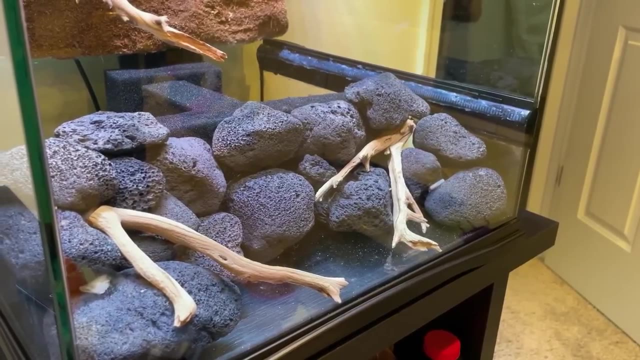 of the cannibal jungle in my bedroom. The tank began as a summer project. I built a custom background for the tank using some ghost wood, spray foam and silicone- Nothing major. The tank wouldn't be the same without it. I built up some lava rock in the foreground. This was to create 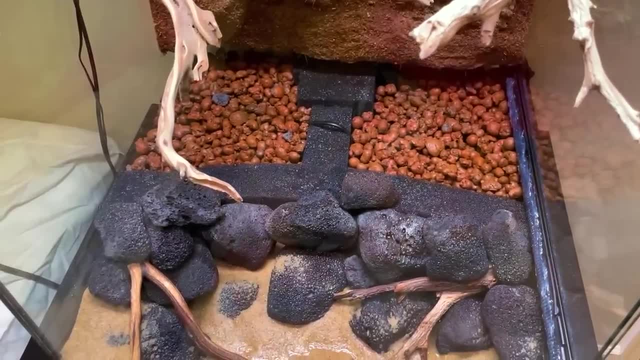 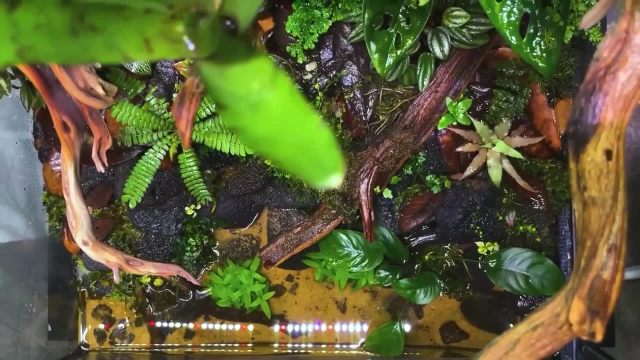 the water area. The back of the tank was then filled with some leca and substrate From here. I planted the tank and it was complete. I didn't realize I had created the groundwork for an ecosystem. At the time, the only animals were these tiny garden snails that hitched along one of the 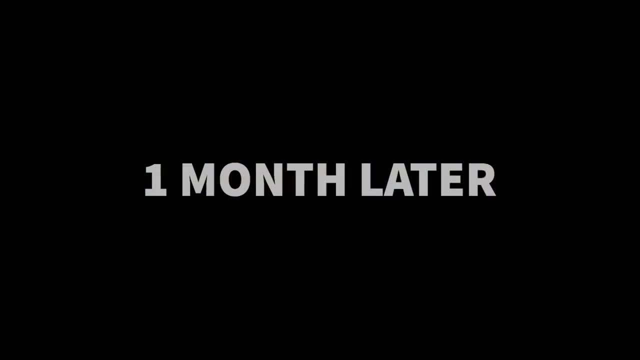 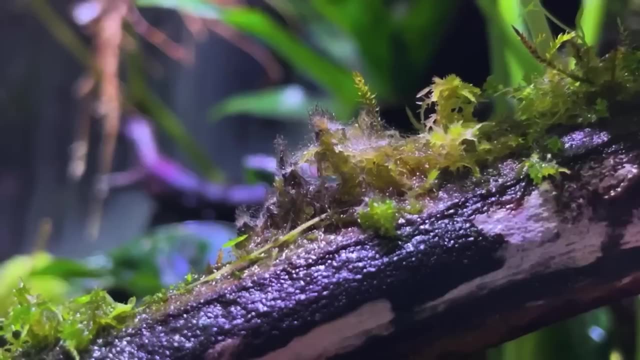 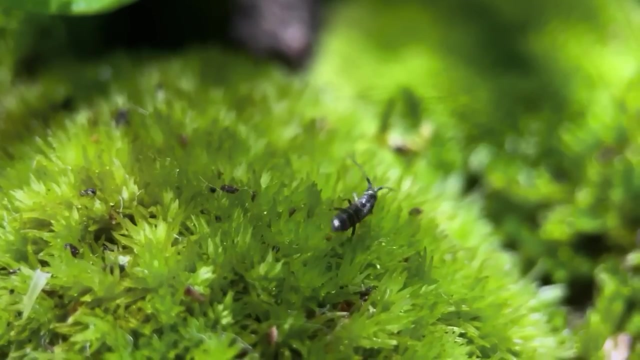 plants. As time went by, the plants started to grow in and moss began to appear. The progression of the tank was slow but clearly evident. Once mold appeared, I introduced various species of springtails into the tank. They thrived in the humid environment. I felt the tank was ready for. 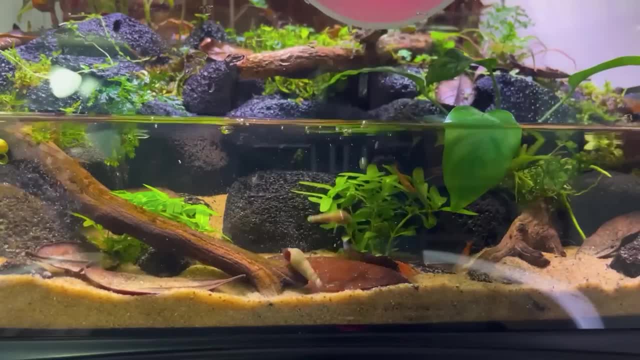 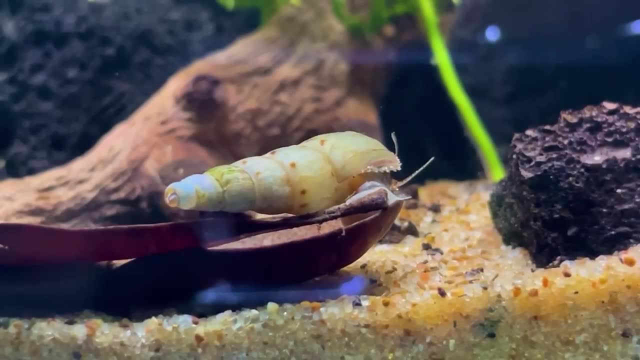 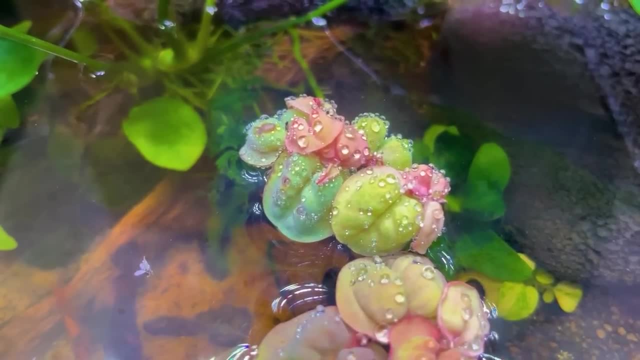 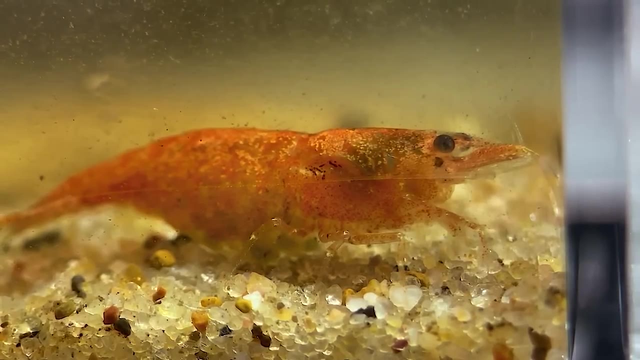 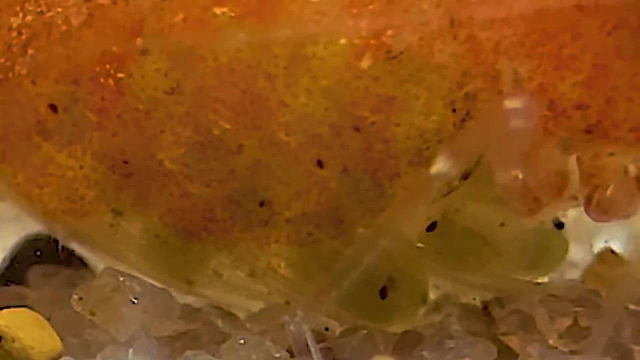 I added in some redroot floater. These plants acted as cover and made the shrimp feel secure. After that, it didn't take long for the shrimp to get busy. Here you can see a very pregnant shrimp. She carries the eggs under her abdomen and those tiny black dots are actually eyes There. 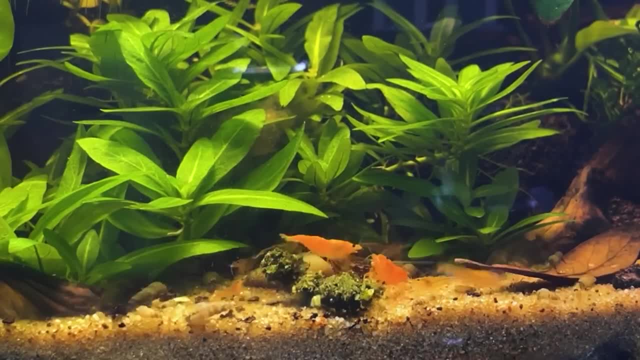 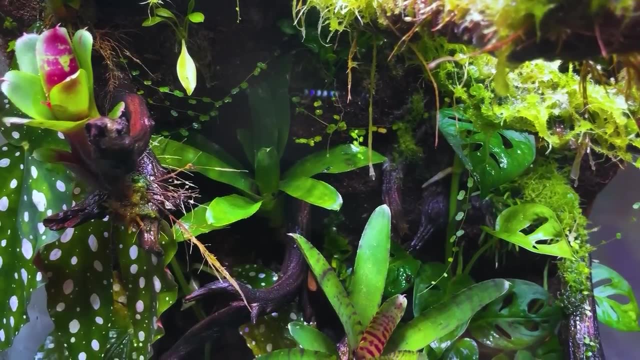 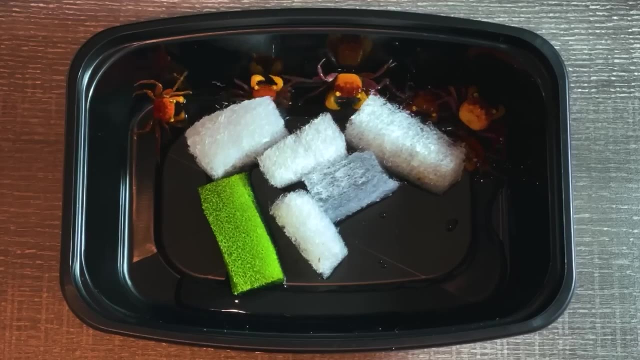 was a population boom and you could clearly see that in the time lapse, About a month down the road, everything was still going smoothly. so I was ready to add in an apex predator, the vampire crab. Their eyes glow a menacing yellow, which is how they get their name. I started with only six of them. 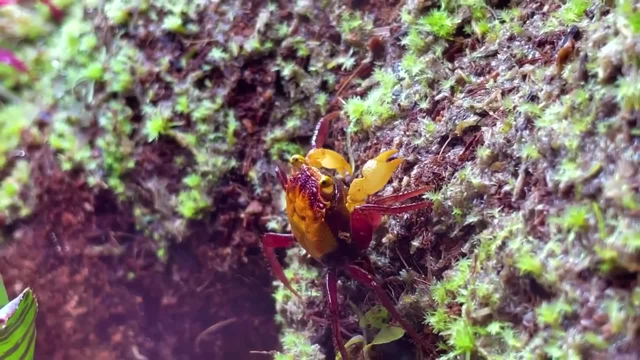 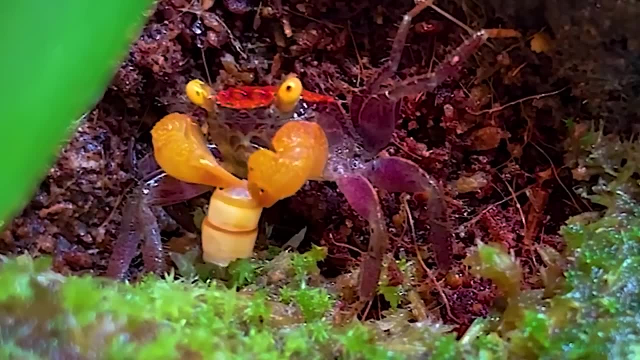 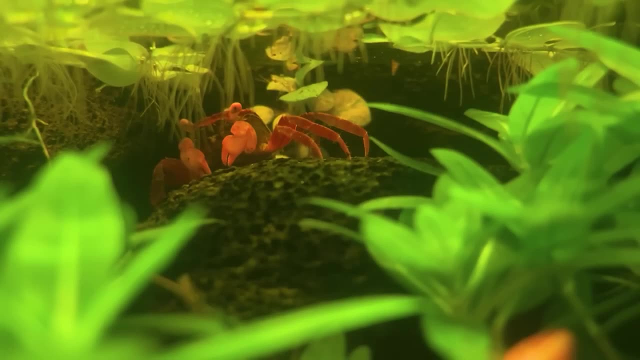 When I added them to the tank, little did I know of the army they would become. I gave them each a mealworm to feed upon. This crab eats his food like a cup of takeout. I always thought it was funny. These crabs are semi-terrestrial, meaning they need both a land and water area to survive. 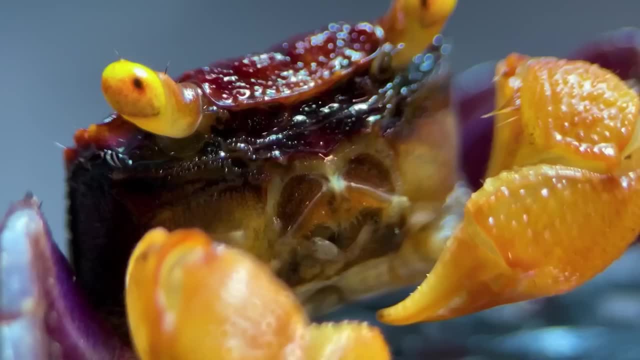 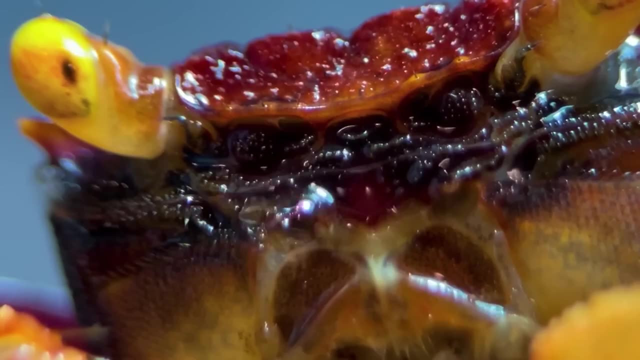 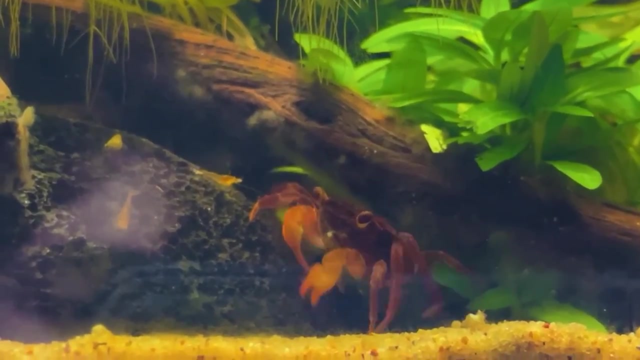 On land. they breathe using a thin layer of water on their shell. If you look closely, you can see the water moving around their exoskeleton. This one is even blowing bubbles. The crabs often venture to the water in search of a meal. They tried to hunt the shrimp, but 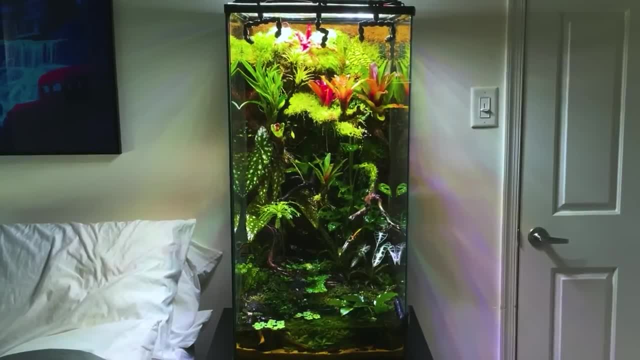 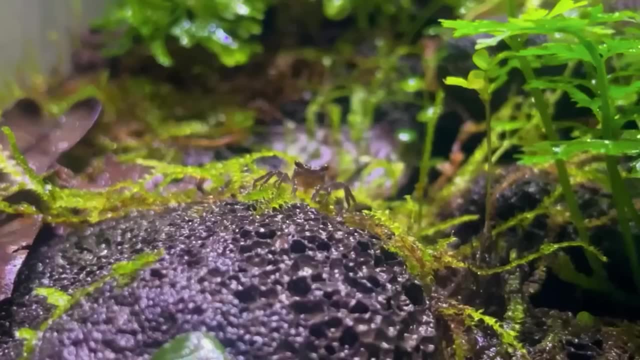 aren't very successful. Two months later, the tank was still thriving. The plants finally started to fill in the space and some of them developed crazy colors. One day I was baffled when I found baby crabs wandering around the tank. They weren't much bigger than a sesame seed. 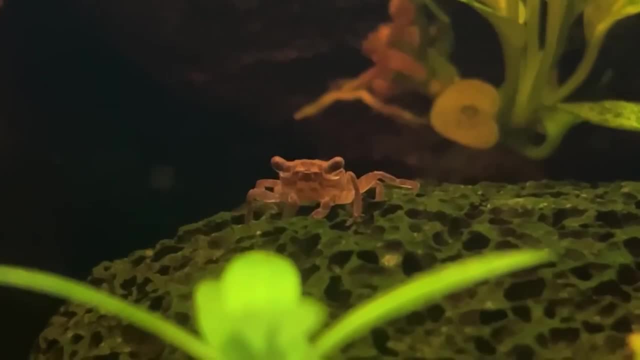 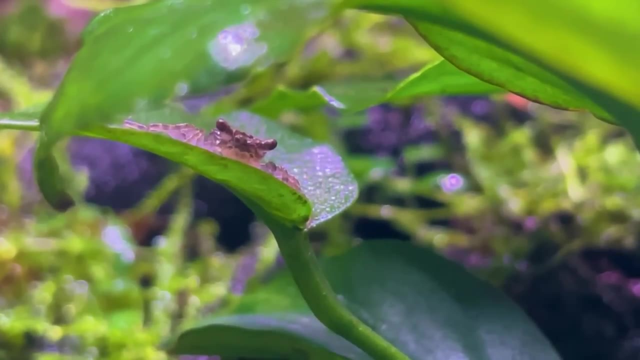 The babies had very effective camouflage as they blended right into their surroundings. Here you can see them eating some algae. The babies were an awesome surprise, though I became concerned. I feared the crabs would overpopulate and there would be way too many. 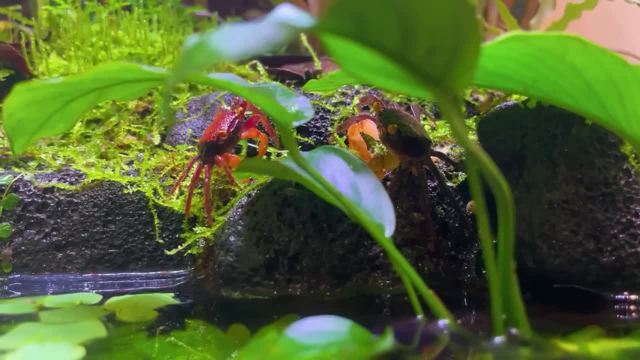 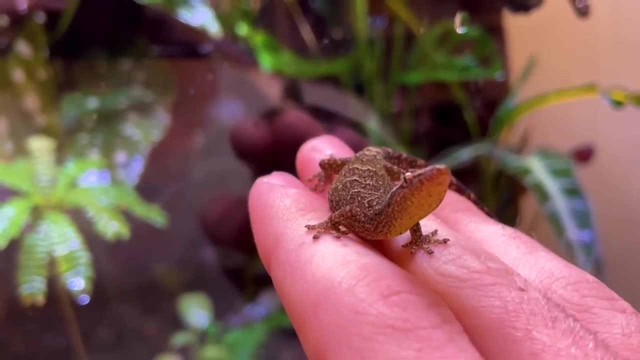 of them. I needed a solution. I needed a new predator. That is where the morning gecko comes in. I bought three adult females and I thought they would be the best prey for me. The geckos immediately took up residence in the canopy. The adult crabs were too big. 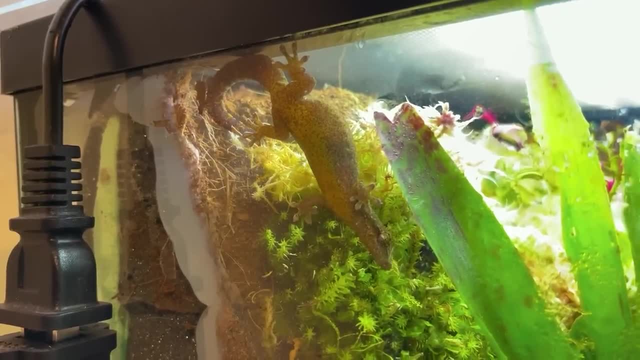 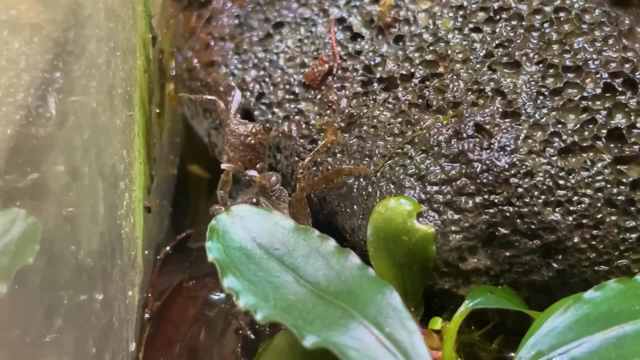 for them to hunt, but the babies? well, the babies could become an unfortunate meal. Now it wasn't only geckos that were hunting the baby crabs. The crabs hunted the crabs. Here you can see a baby crab eating his own brother. They were cannibals. It showed how brutal. 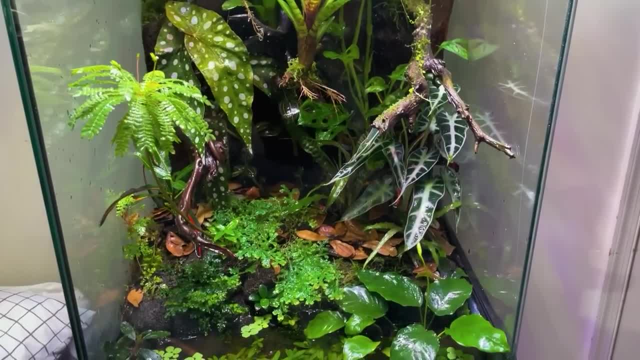 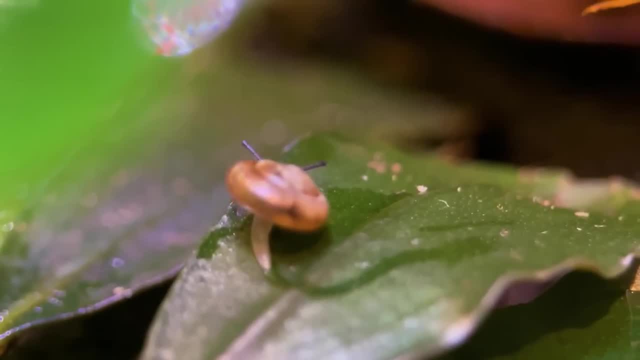 nature can be. As more time passed, the forest floor became much more than just a pile of dead land. The geckos were able to hunt the crabs, and the crabs were able to hunt the leaves. It became a refuge. There were still these tiny snails who would wander in search. 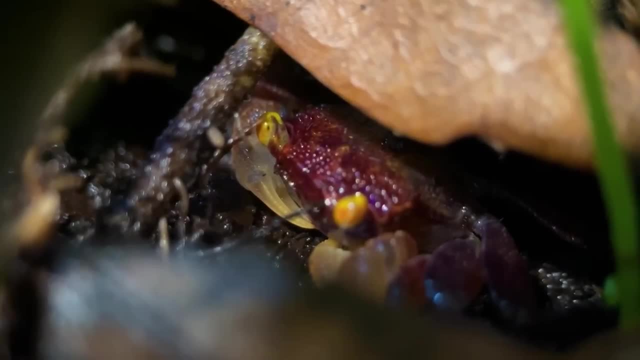 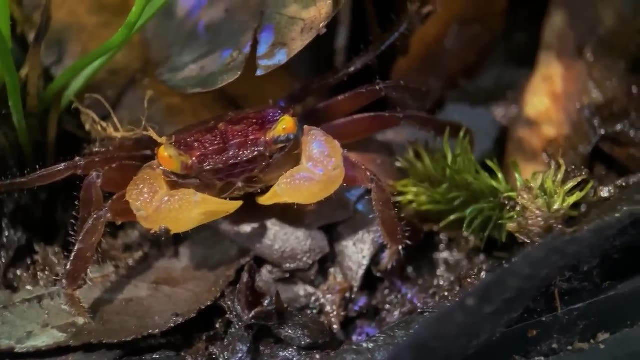 of food. More than just microfauna lived here. It was home to the baby crabs. They rarely ventured out to explore or to become someone else's meal. As the crabs grew, they no longer needed the security of the forest floor. They could climb into the canopy in search. 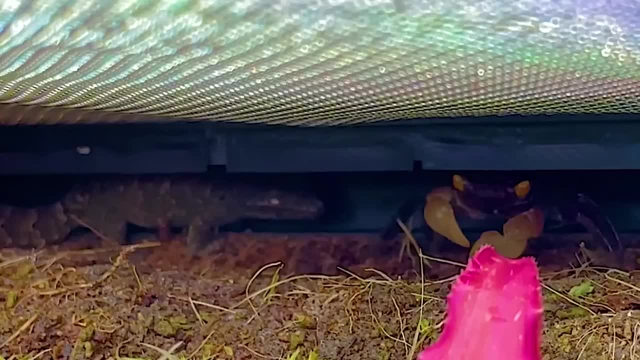 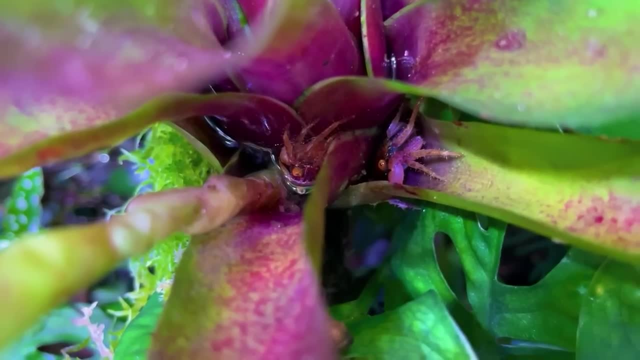 of food. At this stage they were too big to become a meal for one of the geckos. I'd even see them peacefully sitting side by side In the canopy. the crabs found refuge in the bromeliads. These plants hold many pools. 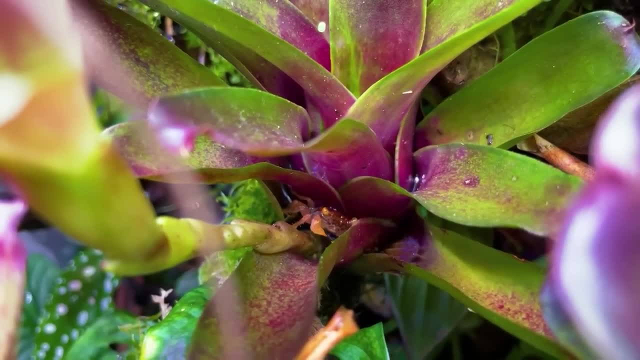 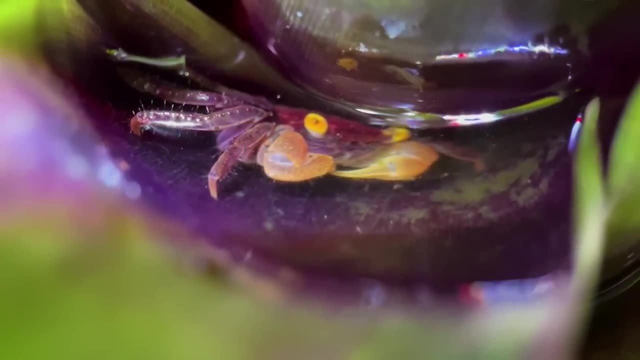 of water in their leaves, which turned out to be a perfect hiding spot. I'd often find them hiding in these pockets. If I ever got too close, they would quickly dive deeper into the plant. The geckos also call the bromeliads home. I'd find them tucked in between their leaves. 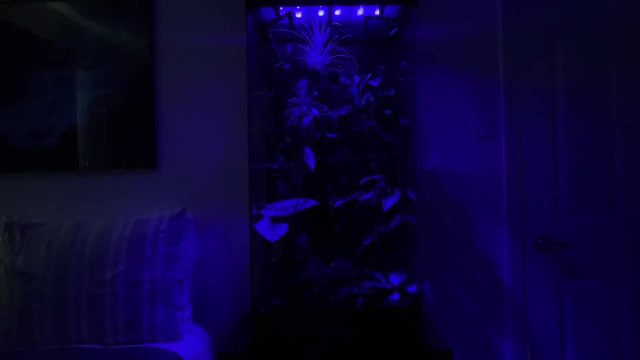 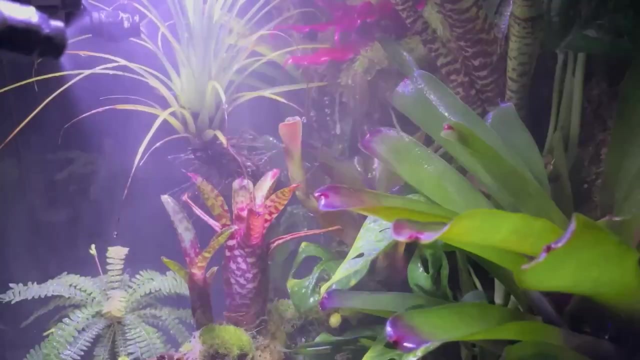 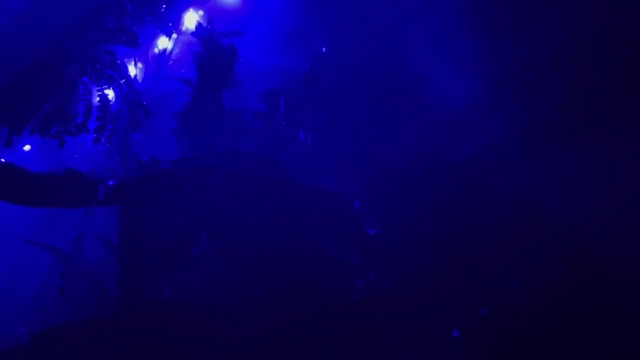 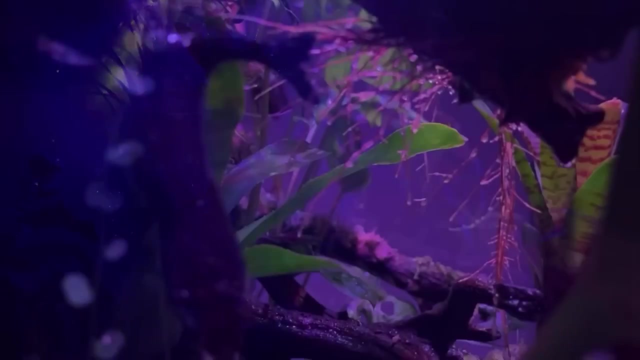 and they'd find shelter here when it rains. Oh yeah, I forgot to mention the tank has rain. The tank has these tropical storms five times a day. The heavy rain brings out the geckos and you can even hear them talking to each other. That clicking noise is actually the 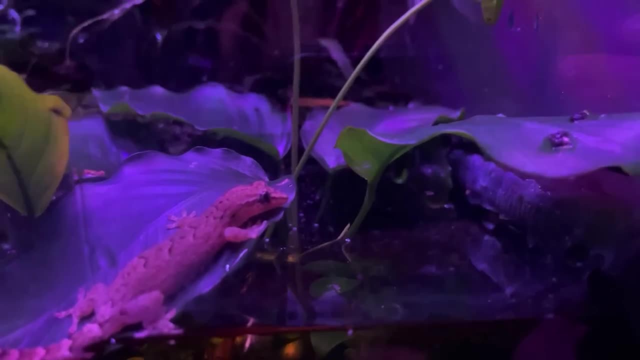 geckos communicating. They are very social animals that like to be housed in groups. Well, their group is about to get bigger because they had laid ponds of food on the ground. The geckos are very social animals that like to be housed in groups. Well, their group. 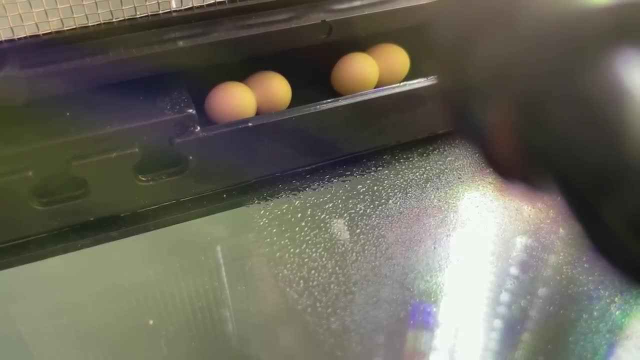 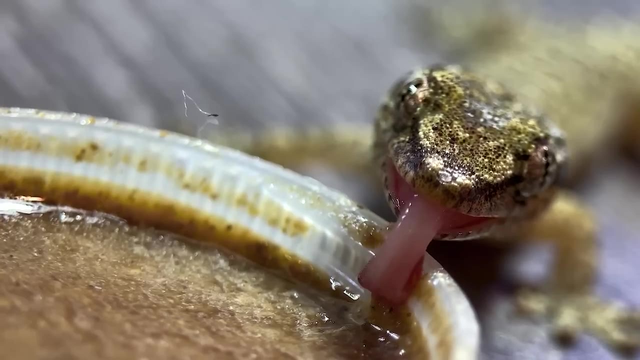 is about to get bigger, because they had laid ponds of food on the ground. They had laid piles and piles of eggs. This may come as a surprise, because if you recall, all the geckos I bought were female, Then how do they reproduce? Well, this isn't just any. 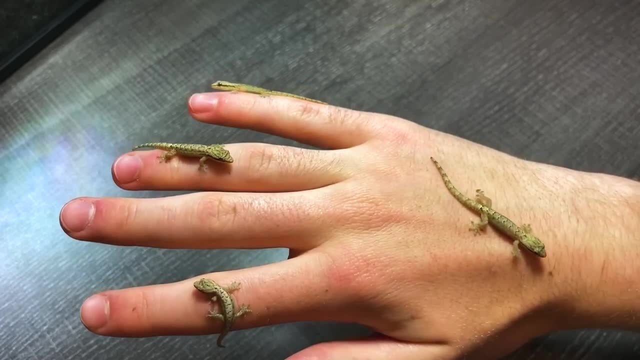 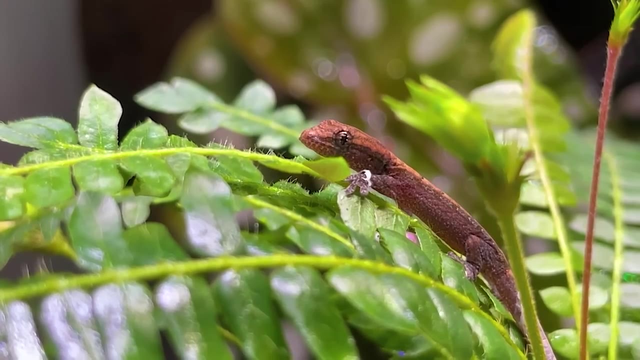 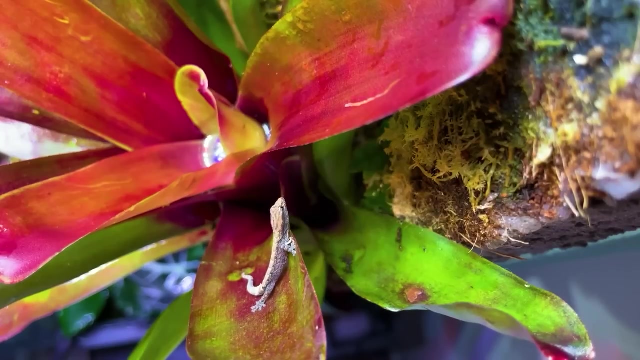 ordinary gecko. This type of gecko can make clones. All you need is one gecko to start an entire population. As the days went by, I began to find baby geckos all over the tank. They were extremely quick and difficult to film. Most of the time I would find them resting among the bromeliads. 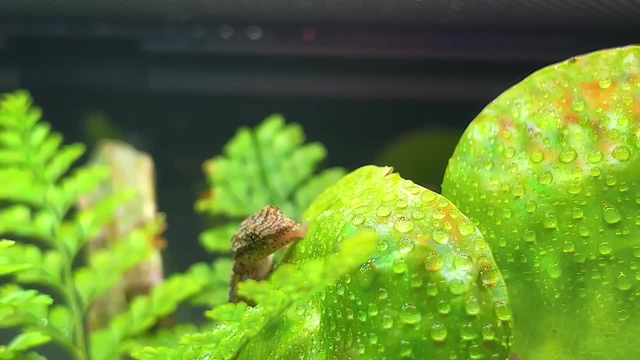 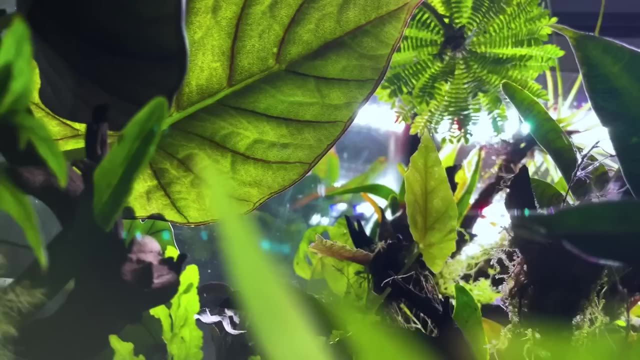 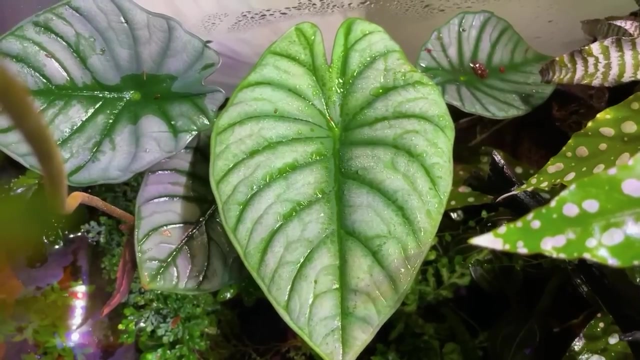 or high up in the canopy, This little guy was drinking off one of the leaves. Funny little guys, for sure. And now this brings us to present day. Like my hair, the tank looks nothing like it did a year ago and has become overgrown. The diversity in leaf shape, size and color is extremely variable. The ecosystem has finally found balance where no animal outcompetes the other. Many of the crabs have reached adulthood. Here you can see a baby, juvenile and adult crab in the palm of my hand. The smallest crab doesn't have any of his adult coloration. 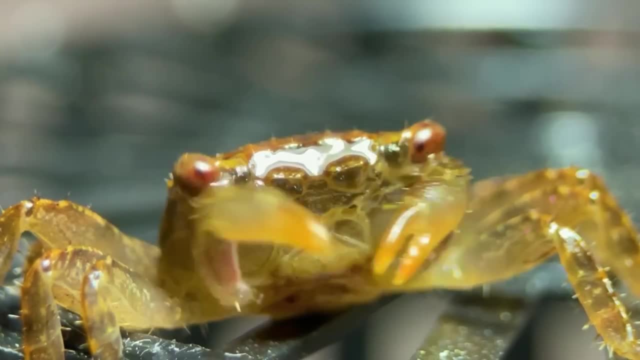 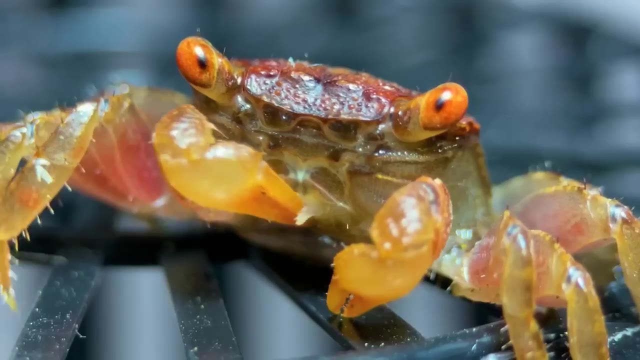 yet Right now he's cleaning his eyes with his claws. They are like mini windshield wipers. because the crabs don't have any eyelids, They have to manually keep their eyes clean. You can see how the juvenile crab has developed some color on his eyes and they're now a